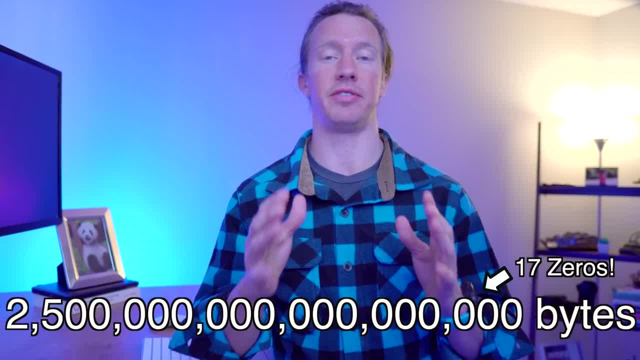 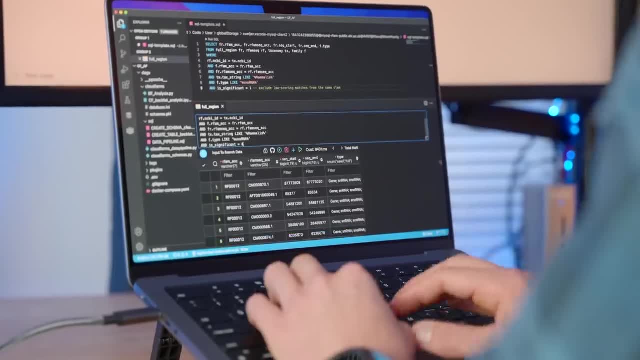 Every day we generate 2.5 quintillion bytes of data, And that's the equivalent of every person in the world filling up an entire Excel file with data every day. And that's where SQL comes in. Developers use this tool to store a lot of the data that we're generating, And then data analysts 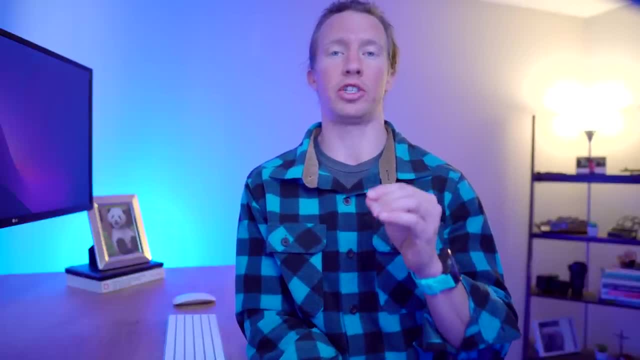 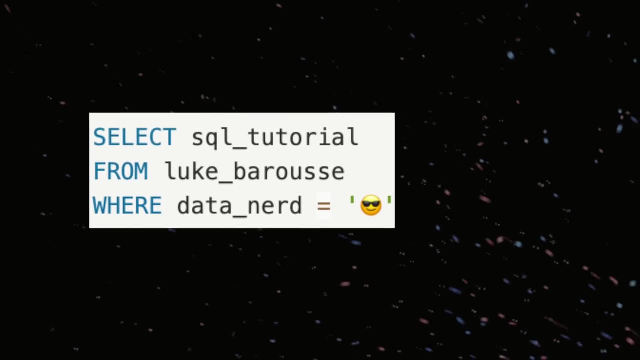 data scientists and even data engineers go in and use SQL in order to access and analyze this data. So let's dive in today to better understand how I use SQL for my job as a data analyst: what is SQL and its importance in working with other data science tools. 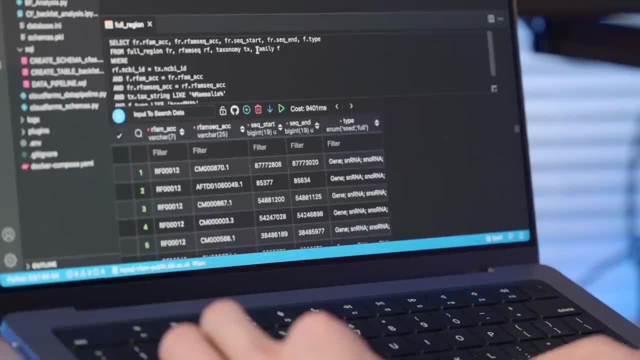 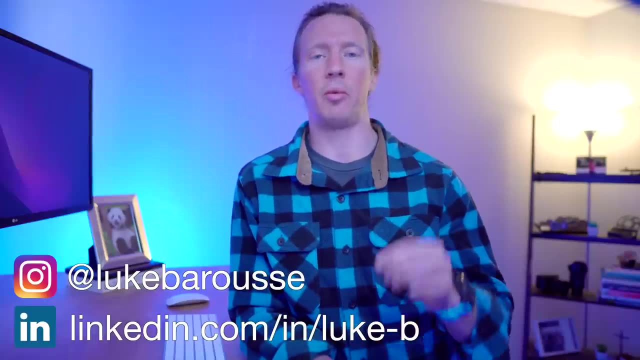 what are the most popular SQL options and by the end we'll even have you up and running with some basic SQL queries. What up data nerds? I'm Luke, a data analyst, and my channel's all about tech and skills for data science And, without a doubt, SQL is the most important tool by those. 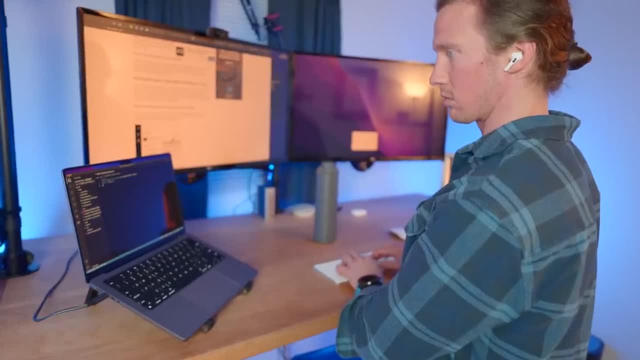 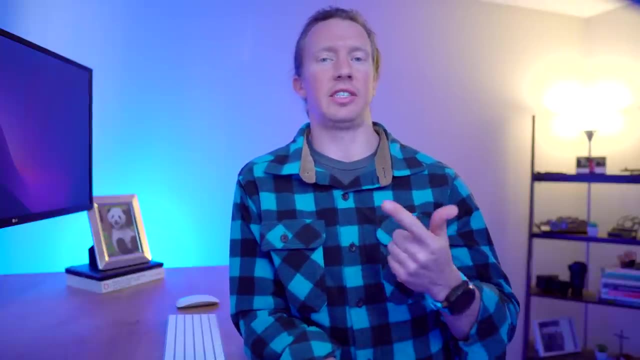 that work in the field of data science. What better way to show this than by sharing how I use SQL in my job, And I find that it's used in two main ways. First is ad hoc analysis and the second is data sharing. Ad hoc analysis of business data is typically performed to answer. 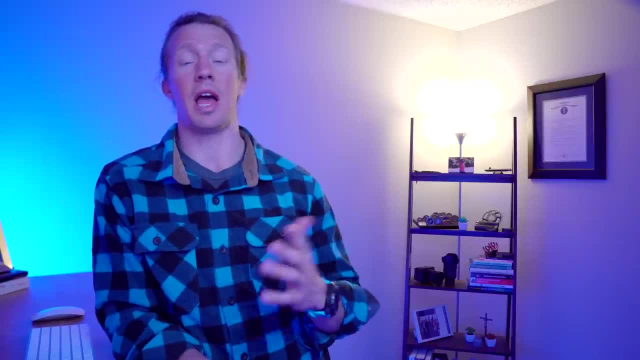 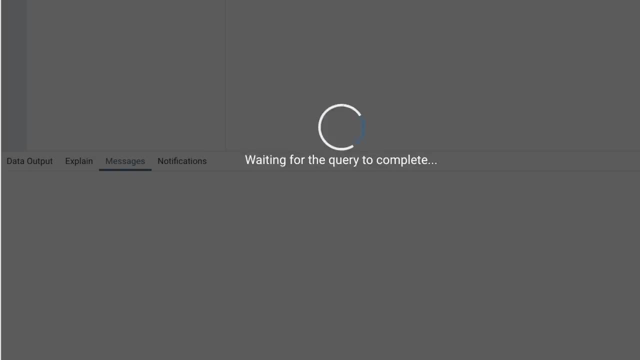 one-off questions. For example, let's say my coworker comes up to me and asks the following: Hey, what were sales last quarter? From here I can use SQL to dive into the data and investigate further, Since I don't need to. 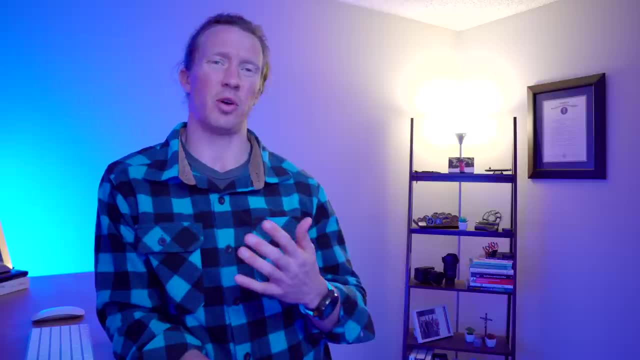 do any fancy reporting. SQL would be fine for this. Now, if my coworker comes back and says this: hey, sales were really low last quarter. Can you look into why this is Now? I could potentially stay in SQL and do this type of analysis, but I found I'm actually more comfortable. 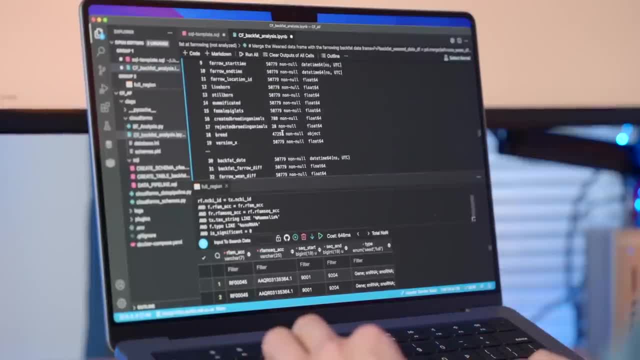 using programming languages for this, So I could use something like Python or R to dive further and investigate further, And I can use SQL to dive into the data and investigate further. So, moving on to that second aspect of data sharing, what happens now? whenever you have a? 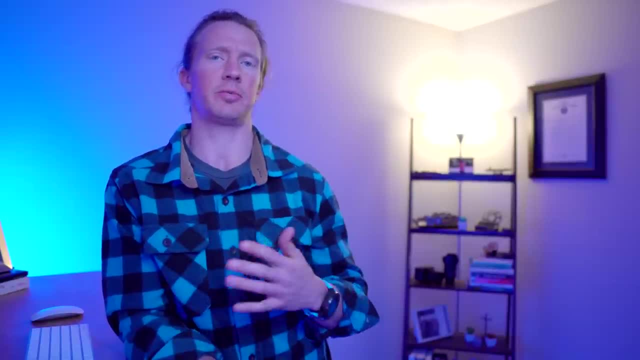 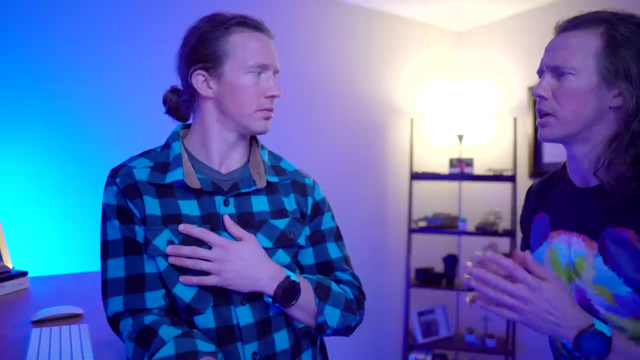 stakeholder that wants to dive into the data themselves. I do expect data nerds to have the skill of SQL, but non-data nerds I don't expect this as much. So you may have questions like this: Hey bro, can I get those sales numbers? but in Excel In this case I could use. 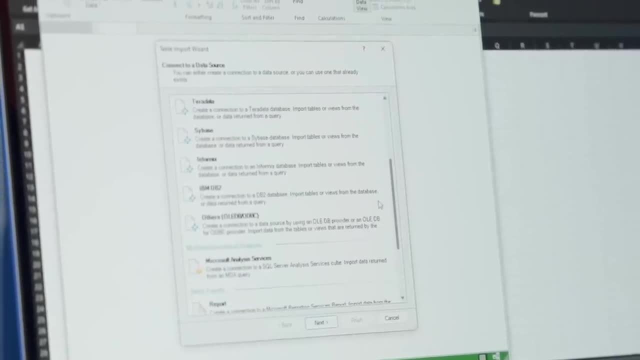 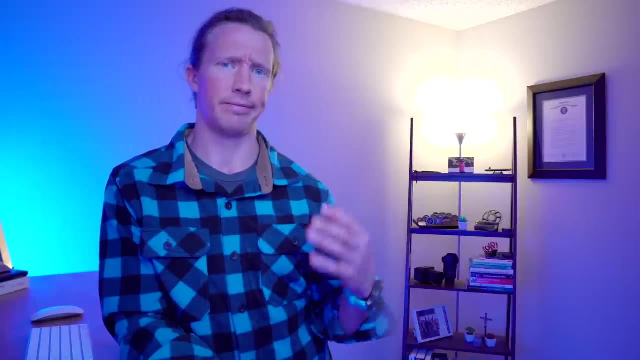 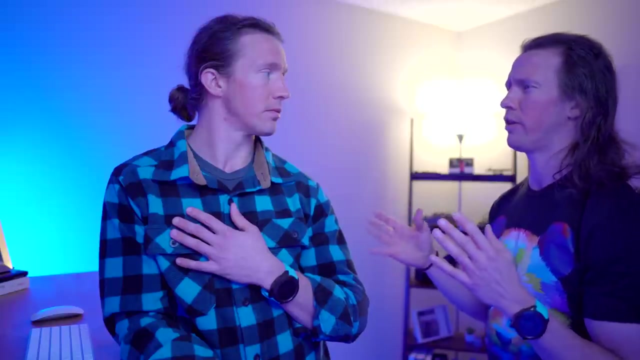 spreadsheet software such as Excel, to connect directly to a database with some sort of SQL code and thus have a live connection to the data within the spreadsheet. What happens if they come back again? Hopefully the final time. And that's the following: Bro, your sales analysis was spot on. Do you mind building a dashboard for the entire sales team? 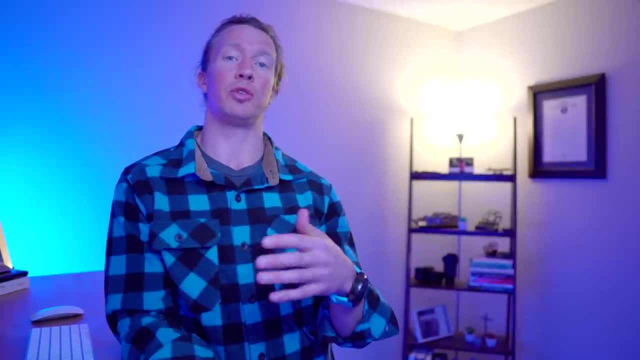 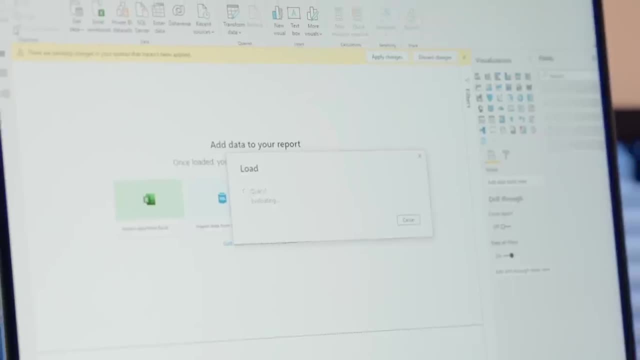 so that way, everybody can monitor this Once again. SQL can be used in visualization tools such as Power BI and Tableau to pull the data real time and display it in a dashboard for my coworkers to admire, And this is why SQL is, in my opinion, the most powerful tool to know as a 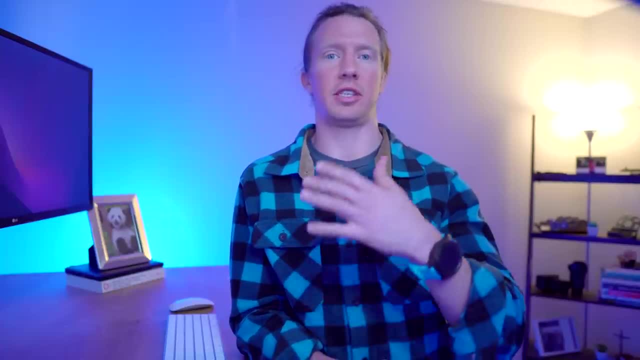 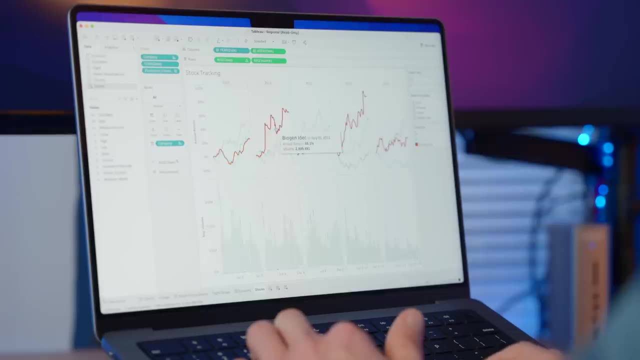 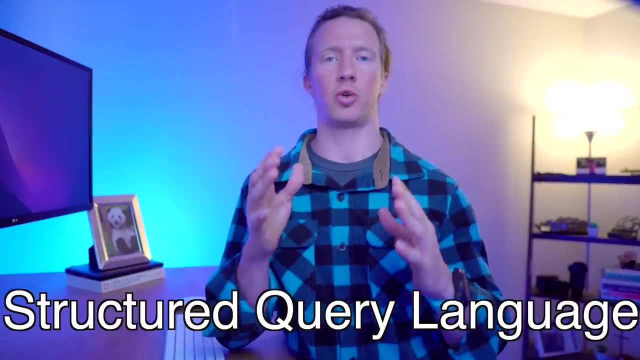 data analyst. Not only can I use this to access and analyze data, I can take it a step further and put it into other data analytical tools to thus extract the data and provide it to my stakeholders. So now let's dive deeper into understanding what SQL actually is. And this stands for structured query. 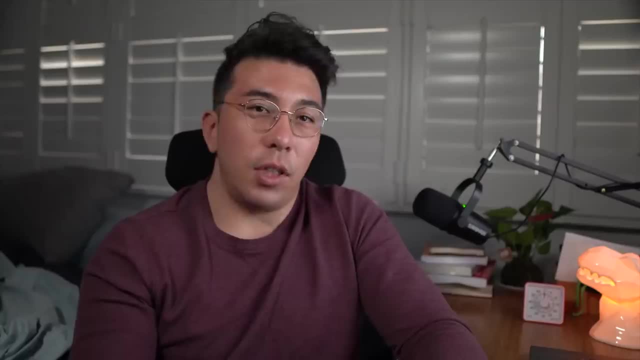 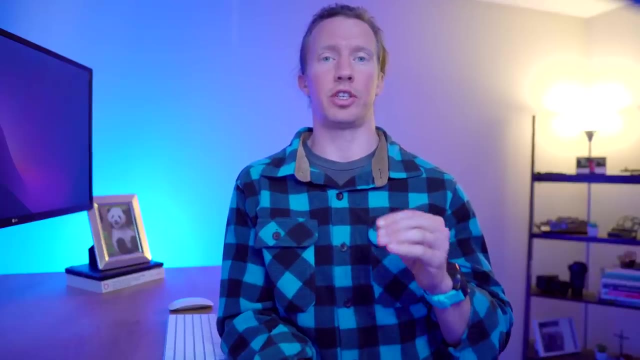 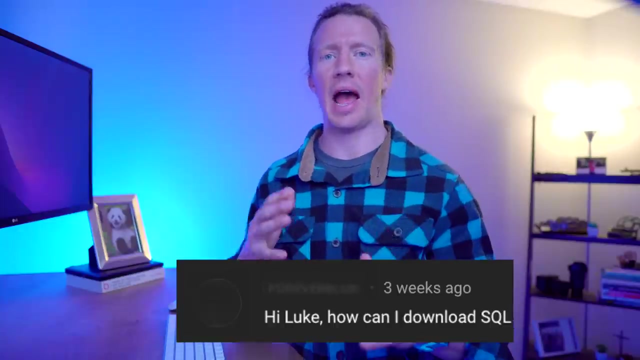 language and its most commonly pronounced, SQL. SQL is the language used to query a database. Basically, think of it like a common language between your computer and a database. So I frequently get asked: how do I? I install SQL on my computer? Now, just to be clear, SQL is a language, so you don't necessarily 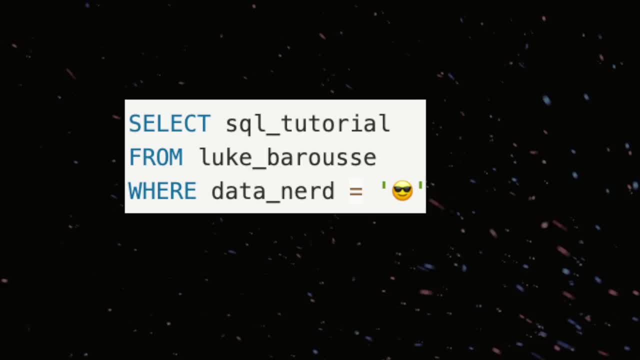 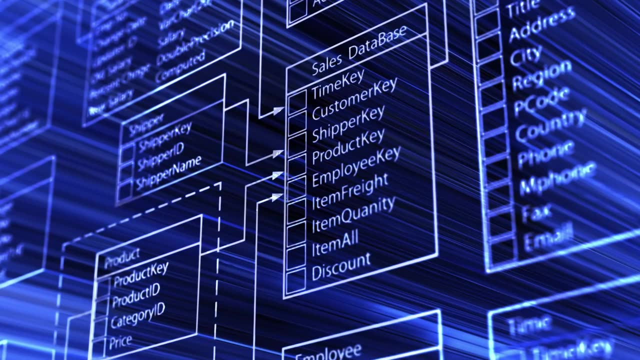 install SQL on your computer Instead. I find that there's two main things that you need to run SQL. One is an editor and two is a database. Let's talk about database first. Databases are an organized collection of data, So large companies use these databases in order to store their vast 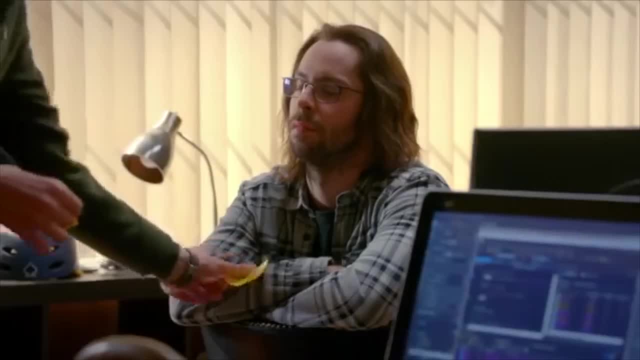 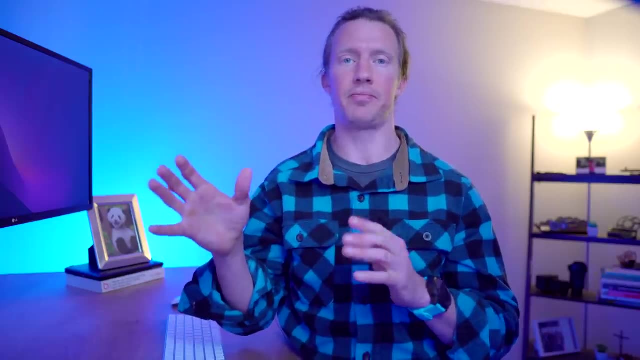 amounts of information. Typically, programmers and even data engineers are utilized in order to build systems around collecting this data. Since we're talking about large amounts of information, we typically don't want to use things like text files or Excel files, because they have pretty 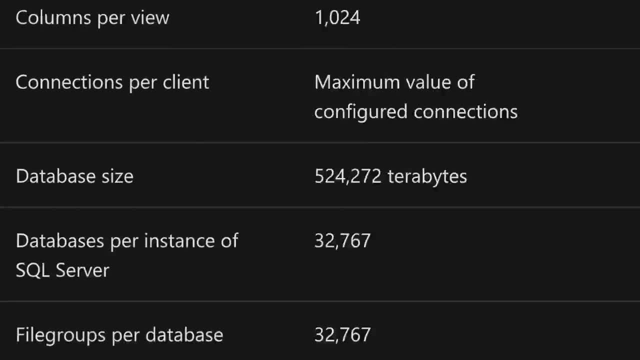 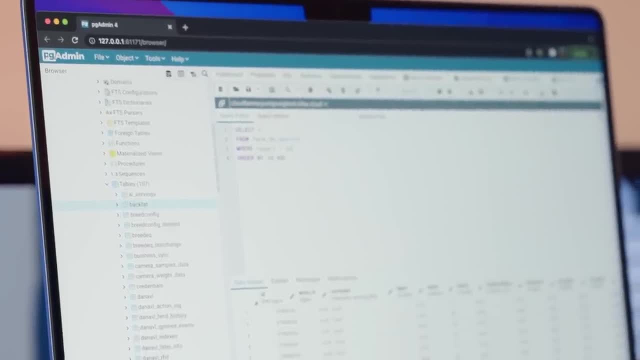 small data limitations. Databases have much larger data limitations. So once these databases are designed and set up by these programmers and data engineers, as a data analyst I can then go in and use SQL in order to query these databases. Now the structure of the language or syntax. 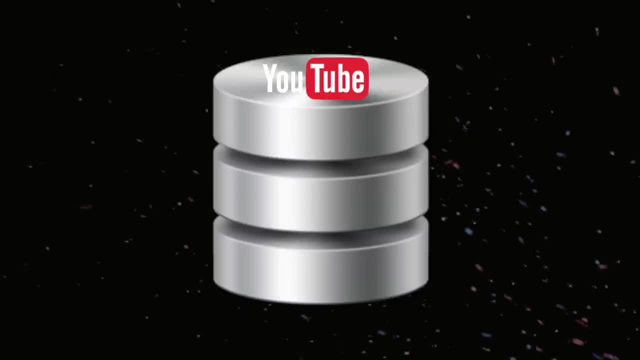 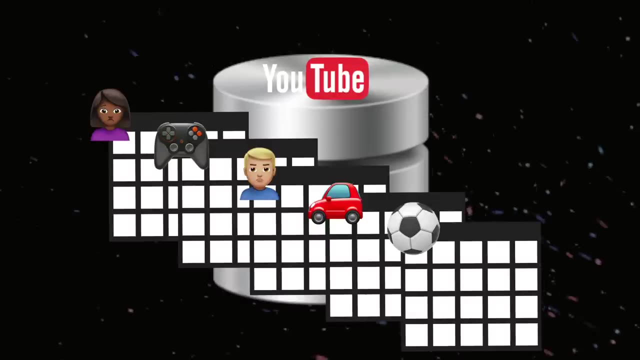 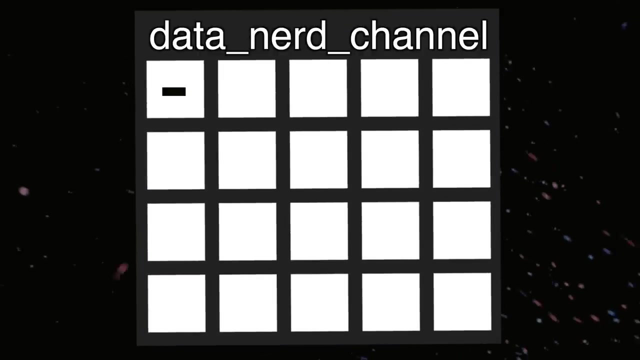 of SQL to query a database is actually quite simple. So let's say YouTube has a database full of information. Inside this database there are different tables for every YouTube channel that include their list of subscribers. We'll say there's a table in there for this channel and it's titled Data Nerd Channel, with an entry for: 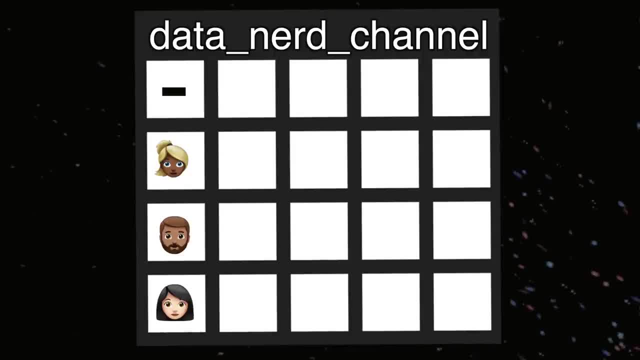 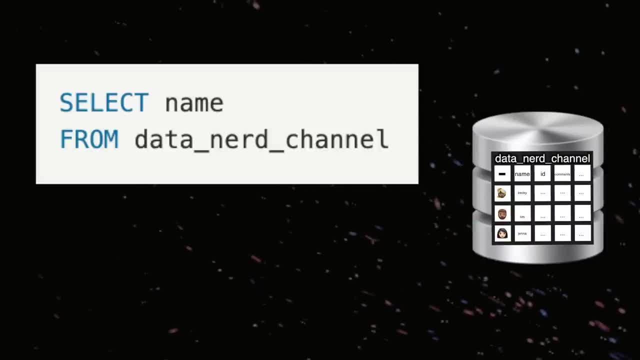 each subscriber of my channel. Each one of those rows in the table has information like name, channel ID and the number of comments they've given. Now I want to get a list of all my subscribers. I then can use the following syntax, which has a SELECT statement and a FROM statement. 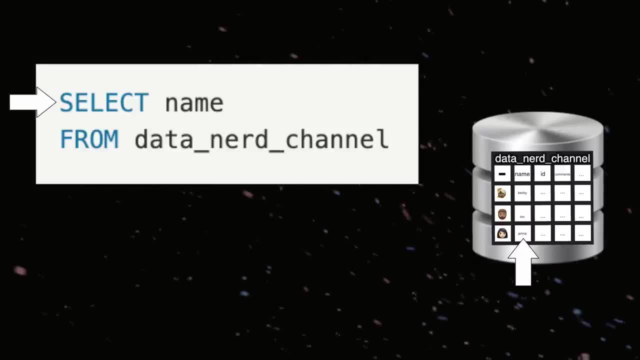 So if I want to get a list of all my subscribers, I can use the following syntax, which has a SELECT statement and a FROM statement. So SELECT is used to identify the column of interest that we want to grab and FROM is used to identify the table we want to connect to When I send this query to the database. 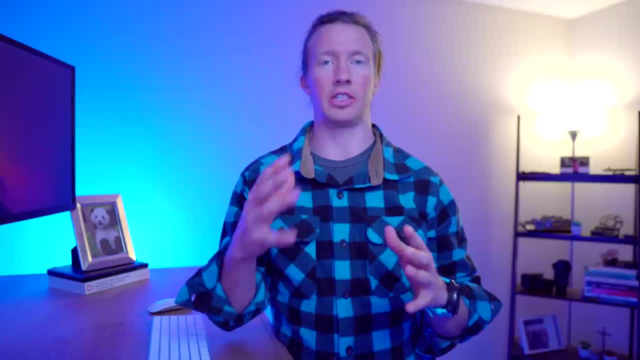 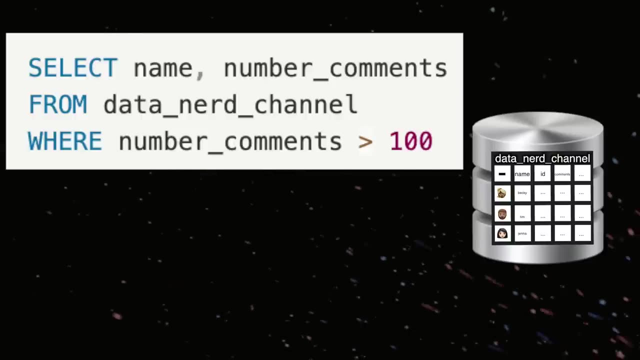 it then will provide me back a list of all my subscribers. Now, SQL can be used in a lot more different ways. For example, we can actually use it to go in further and analyze the data, such in this case, where we can add on a WHERE statement to filter our data further based on how. 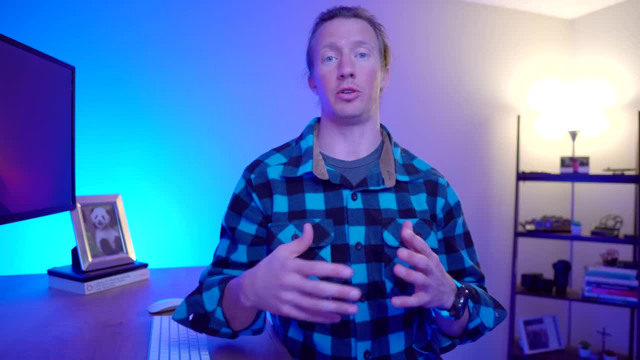 many users commented more than 100 times. We can also use SQL to insert or store more information in a database. So if I want to get a list of all my subscribers, I can use the following syntax, which has a SELECT statement and a FROM statement. For this, we can identify the table and columns. 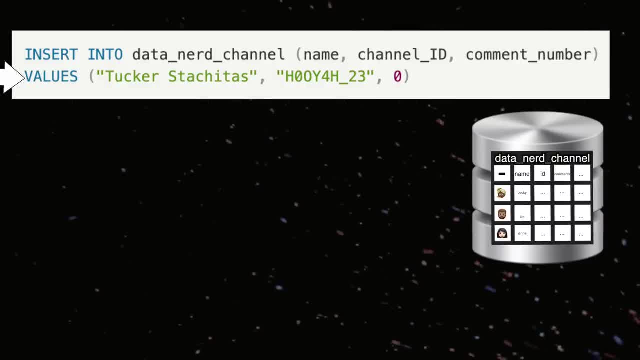 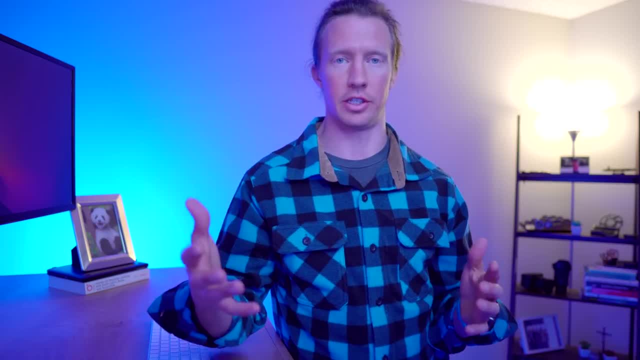 we want to insert into and then provide the values to insert into this table. Once I run this, the table will be updated And then, finally, we can use SQL to update record entries. For this, let's say we have a new comment on one of my videos. Once again, we can identify the table. 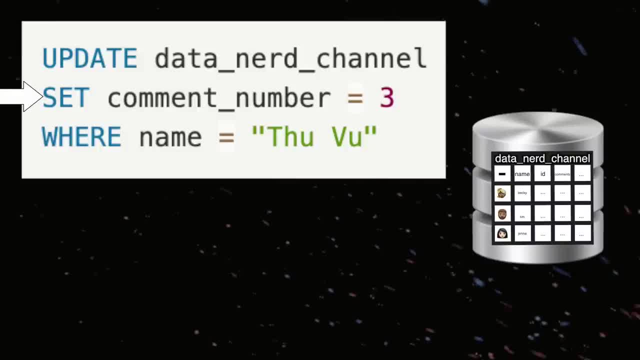 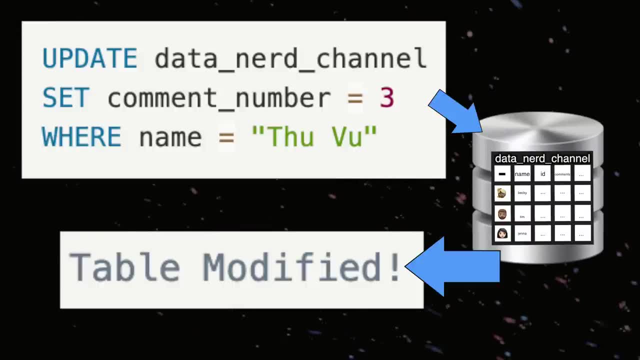 we want to update the column. we want to set a new value for and then a WHERE statement to select what to filter on for that entry. Once I run this, the table will be updated. So now we understand how to query a database and generally what a database is. 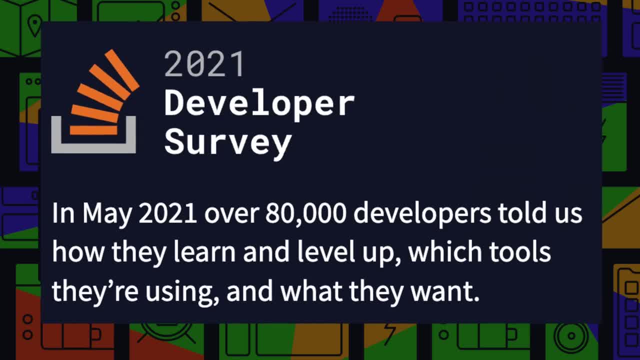 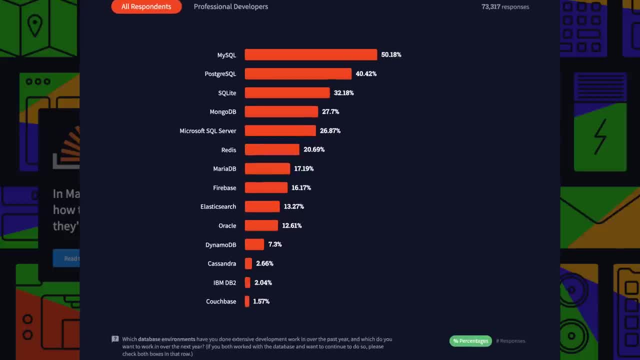 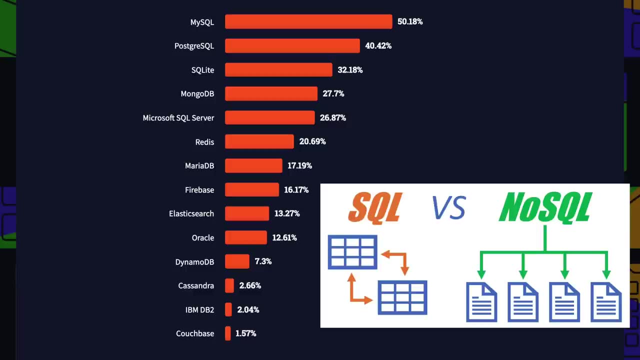 but what database do you use? Well, Stack Overflow conducted a survey last year that asked respondents about what software tools they used for their job. When we look at the most popular database options, we can see that there are a plethora of options to choose from. To make things a little complicated, there's actually two types of databases on this. 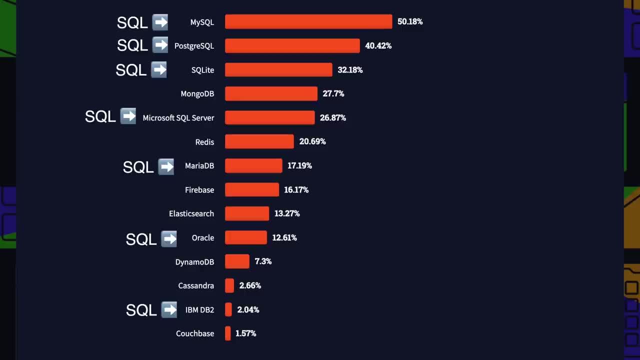 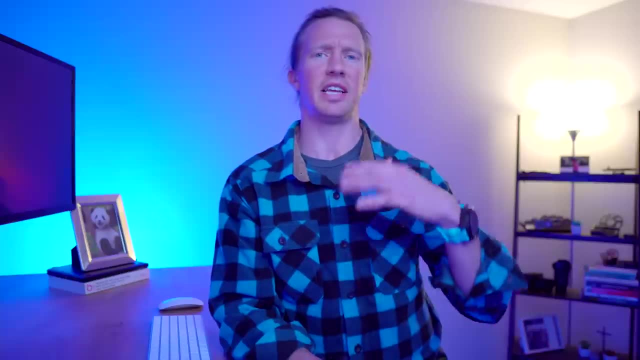 survey. There are relational databases, so SQL databases, and non-relational databases, or NoSQL databases. I'd focus on the relational databases, as they typically store data in a tabular form, which is more common for our job. But what about those NoSQL databases? 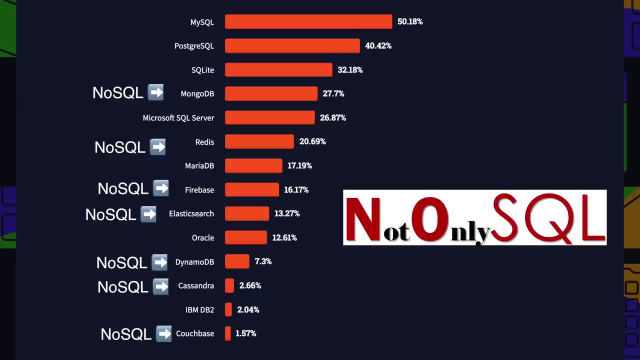 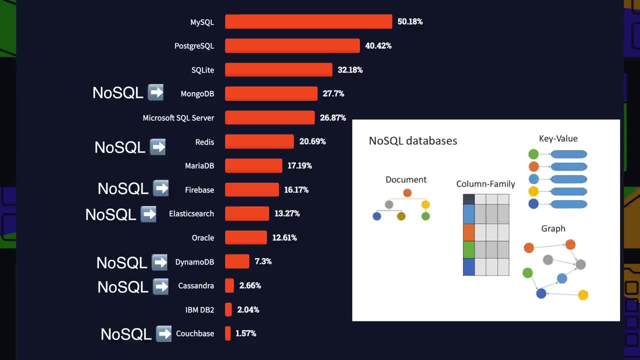 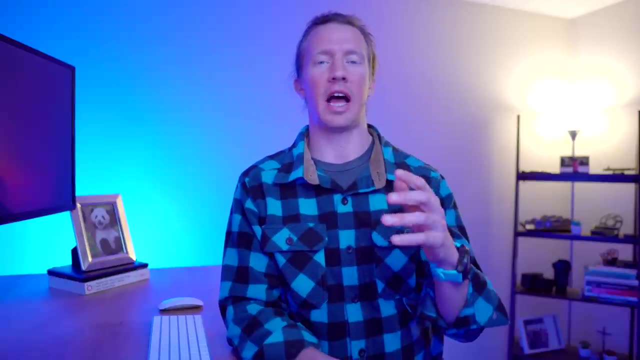 So NoSQL actually stands for Not Only SQL, meaning that you can not only store this data in a tabular form, it also has a manner for you to store it in an unstructured manner, which is actually more efficient at handling very large amounts of data. So for aspiring data analysts, I think it's more. 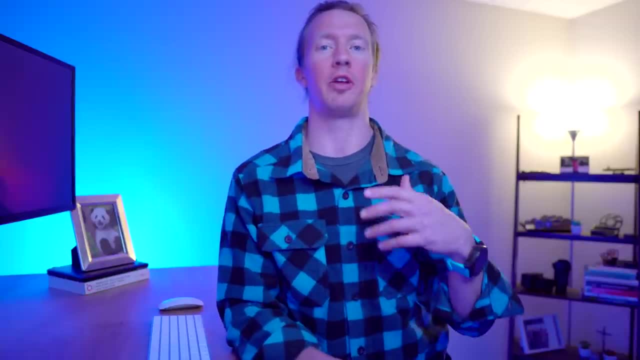 important that you're aware of this. That way, you don't have to worry too much about it. You don't have to worry too much about it. You don't have to worry too much about it. While you progress in your career, you may potentially become in contact with these, and then you can learn about 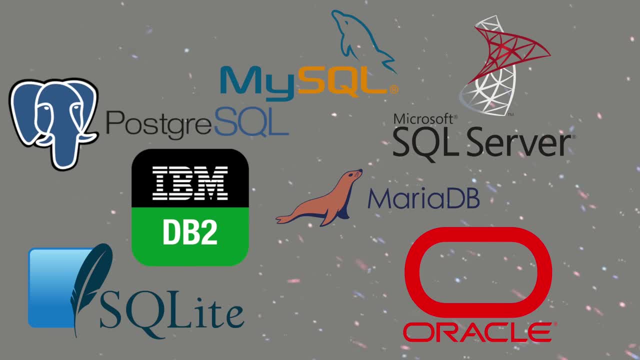 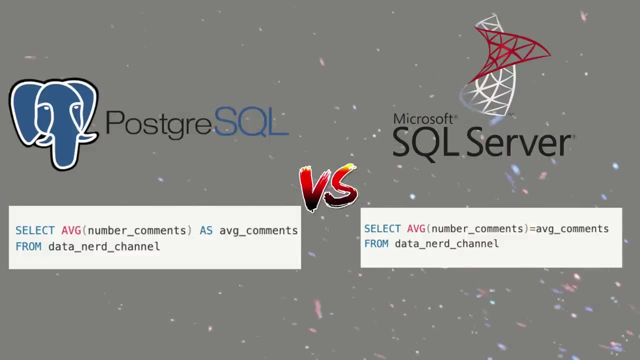 it then. So then, what relational database should you learn or use? Well, quite honestly, I don't think it matters, as all of these relational databases use the same SQL syntax and you can transfer your skills between them. But, interesting enough, the most popular options on that Stack? 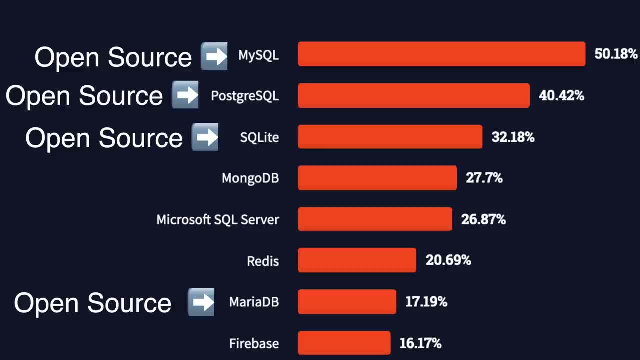 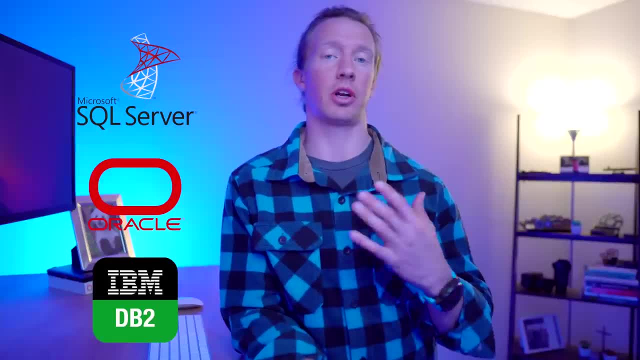 Overflow list are also free and open source. So I would say, start with any one of these. Personally, I use Postgres and also SQLite for all my consulting projects. The other options are closed source and not always free, although they are very popular. especially they're being 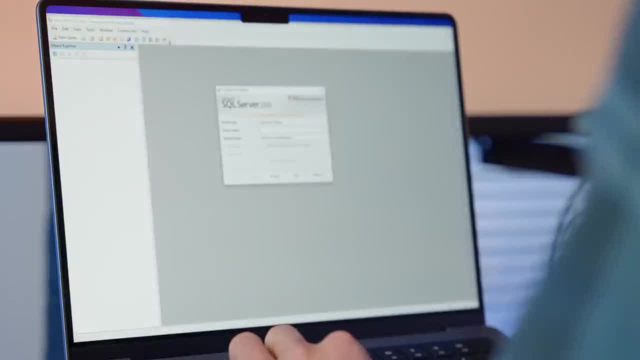 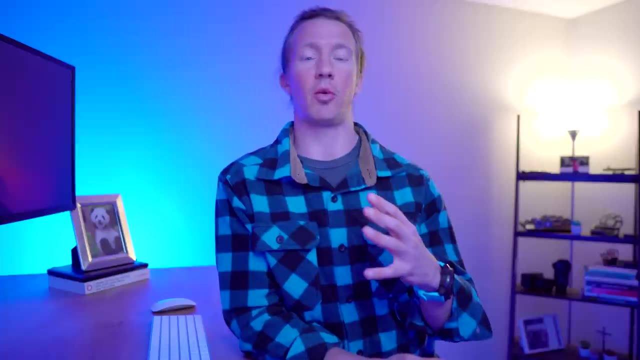 used in large corporations. Of these options, I've used primarily SQL Server for all of my work projects. This is also great because this choice has a free option available. Having worked with a lot of these different databases, I can say it's with pretty relative ease that you can switch. 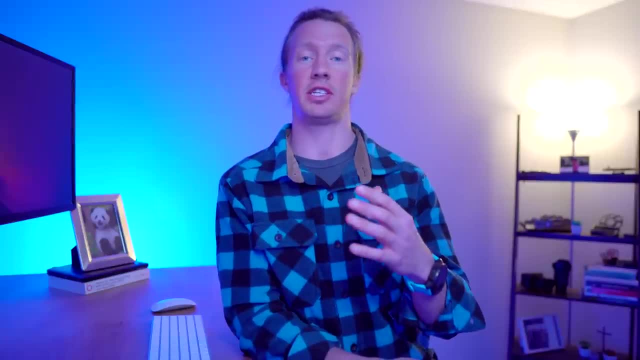 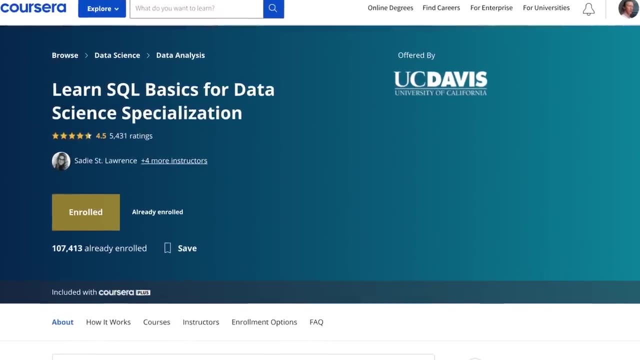 between them. The hardest part is learning the basics of the syntax for SQL. So all this actually directly relates to the sponsor of this video, Coursera. My favorite Coursera sponsor is Coursera. My favorite training for this on Coursera is the SQL for Data Science specialization. 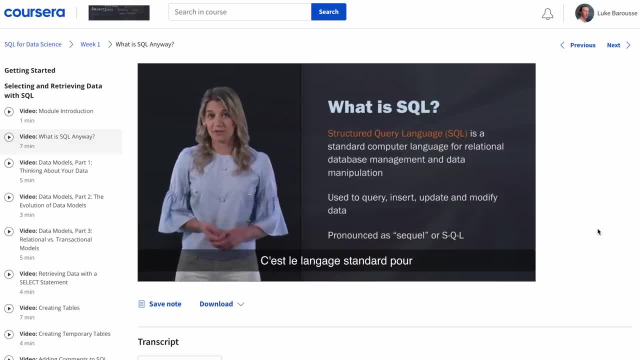 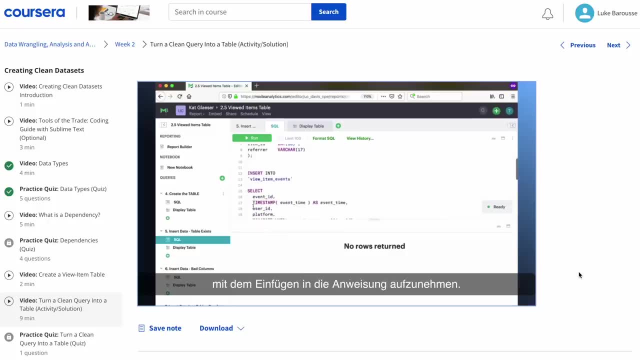 which is perfect for those that have no prior experience with coding, that want to master SQL. I even think it's great for those that have already obtained, maybe, the Google Data Analytics certificate, because now that you have these basics of SQL, you can use this specialization to dive. 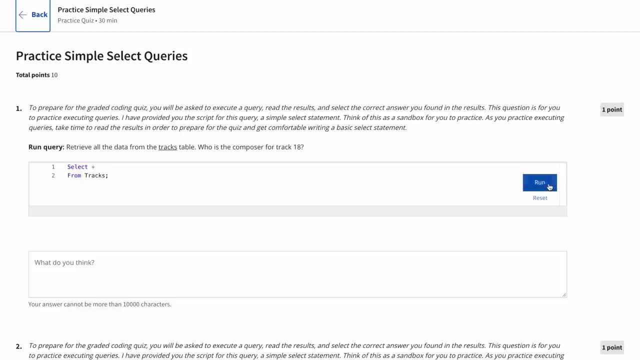 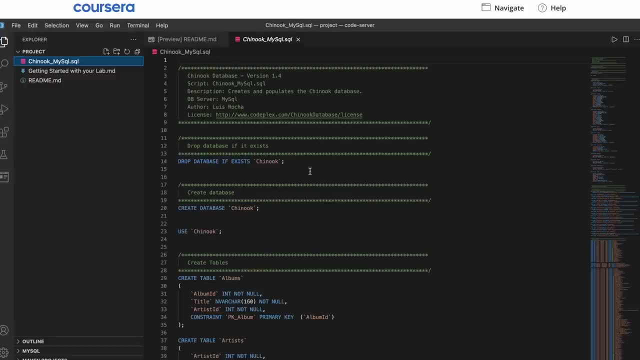 further into it. The course focuses on SQLite, and what I like about the platform that Coursera provides is that they get you up and running with the same tools they'll be using in real life without having to install the same tools they use in the real world, So that's a great thing to do. 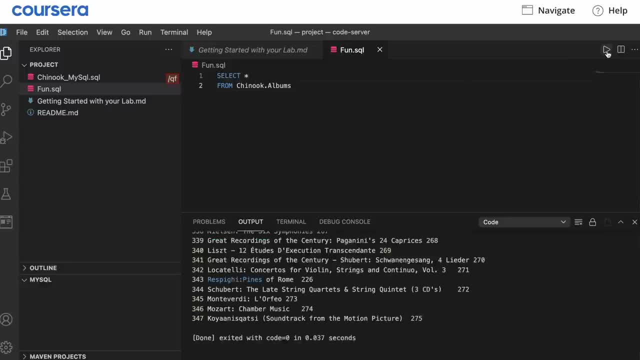 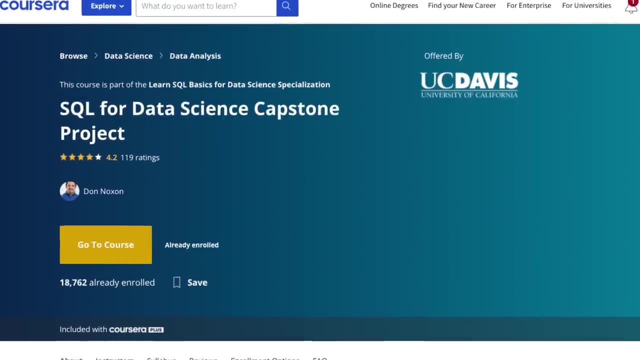 For example, I use VS Code for all my coding, in both Python and SQL. I also like how the specializations have a capstone project, So you can then take all those skills that you've learned over the courses and apply them into a final deliverable, which you then can use to showcase. 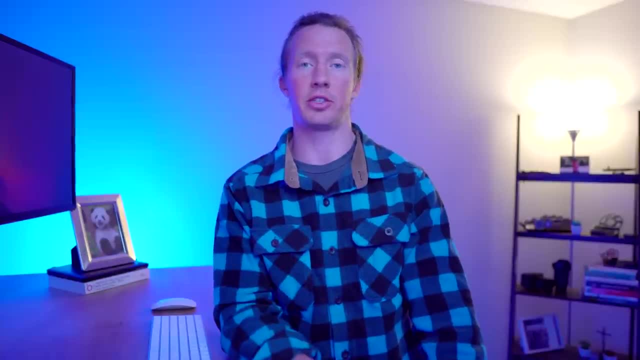 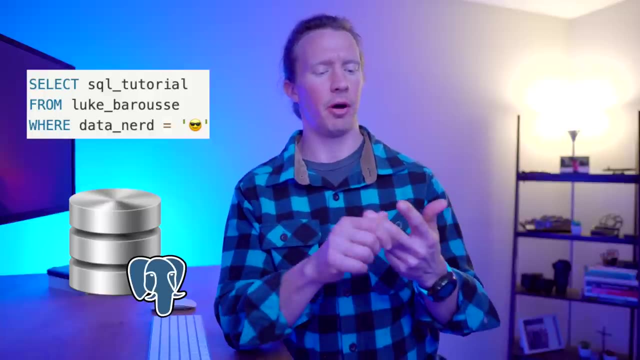 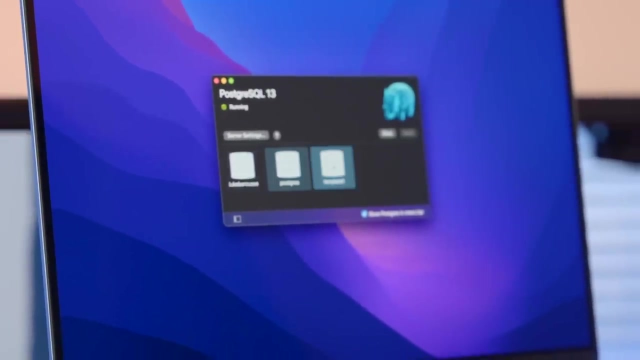 on your resume as experience. So thanks again to Coursera for sponsoring this video. So we talked about already SQL syntax, also about databases themselves. but where do we keep these databases that we're trying to query? Well, the first option is that you can keep the database locally running. 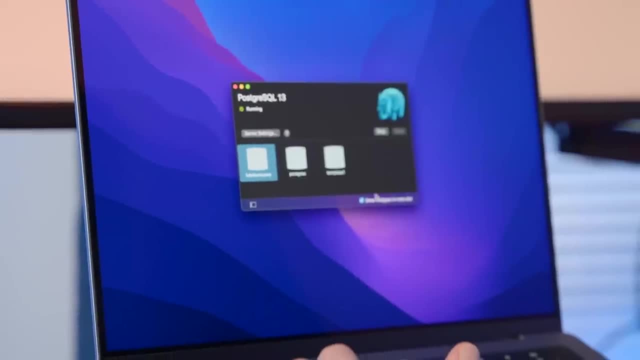 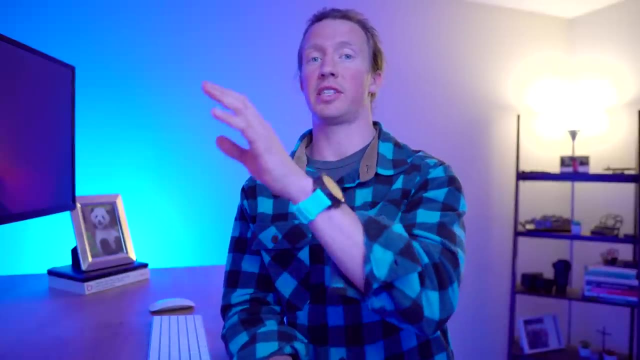 on your computer, And this is a great option, especially if you're learning or you're new to SQL. It very much simplifies things. Now, sometimes I'm even doing data analytic projects that need access to a remote database, and sometimes the owners don't want you to have access to it. 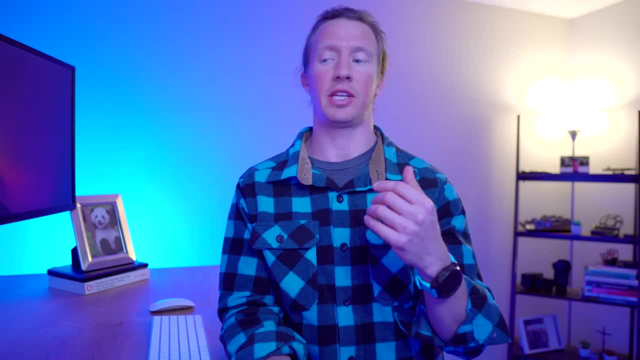 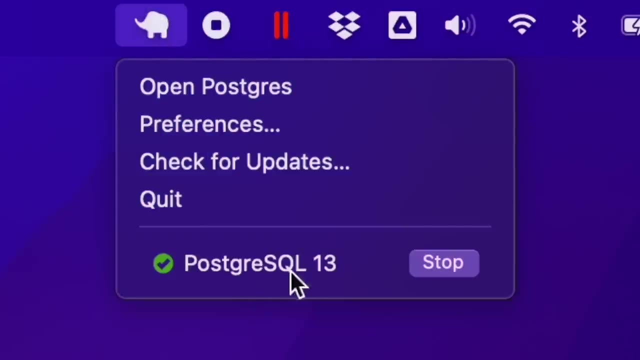 So in that case I can download a copy of that database and have it running locally on my computer. I do this most frequently with Postgres databases, So because of this I have the Postgres application installed on my computer so I can run these databases locally. This will be the 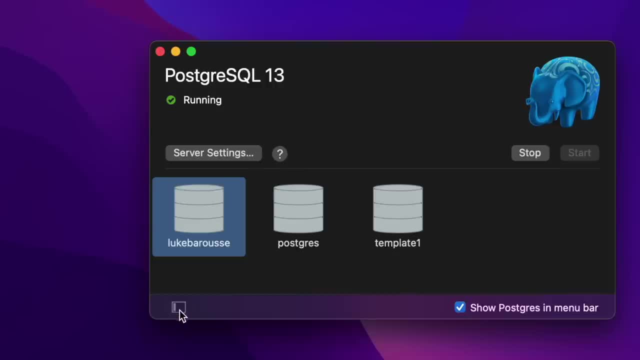 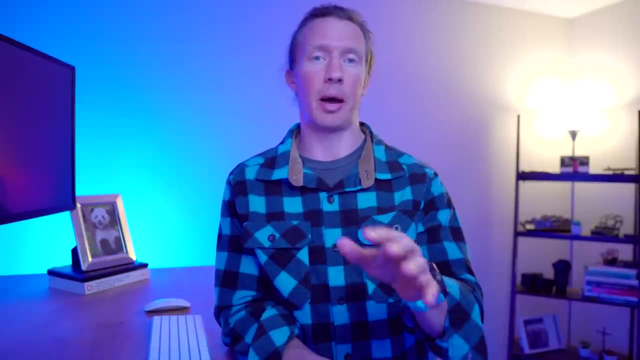 same for any other popular database. Now, running a database locally on a computer is a great option if you're the only person accessing it. Once you get into other people accessing it, you need to look at other options. So the two popular options for this are some sort of server or a cloud. 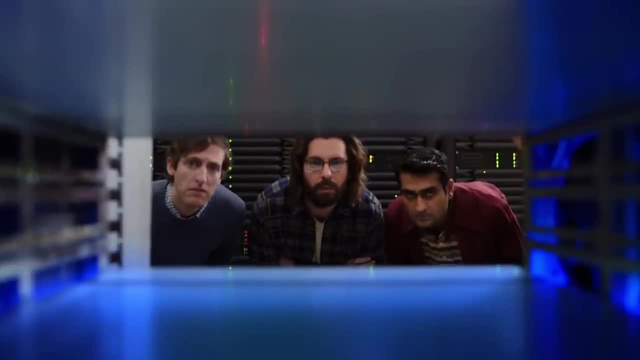 provider For the server option. many large companies have their own where they like to store their own data. Typically, your IT department will handle installing and setting up all the dependencies for the database, So if you have a server that you're not familiar with, you can. 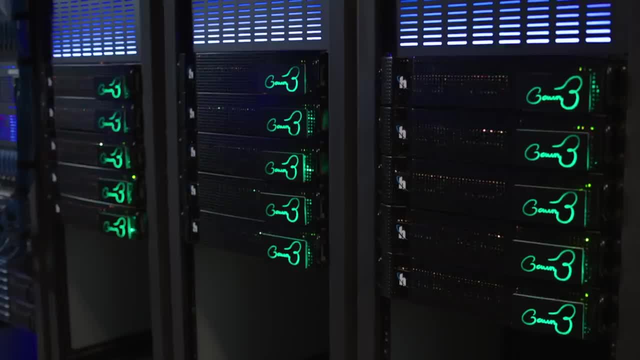 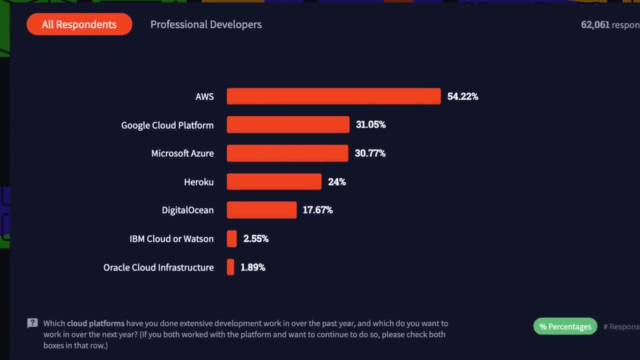 download a database and then grant you access. This option is called on-prem. Now, another popular option is to use a cloud provider instead. Looking back at the Stack Overflow poll, the most popular options are from Amazon, Google, Microsoft and even Heroku. 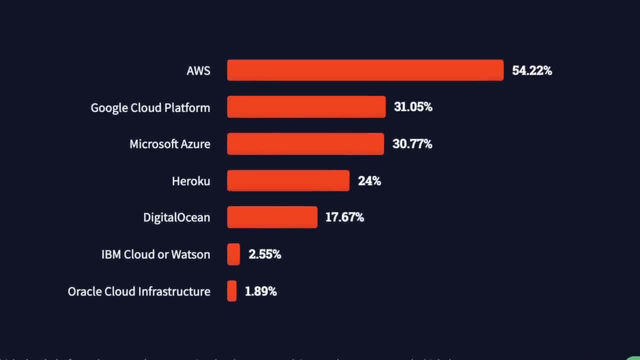 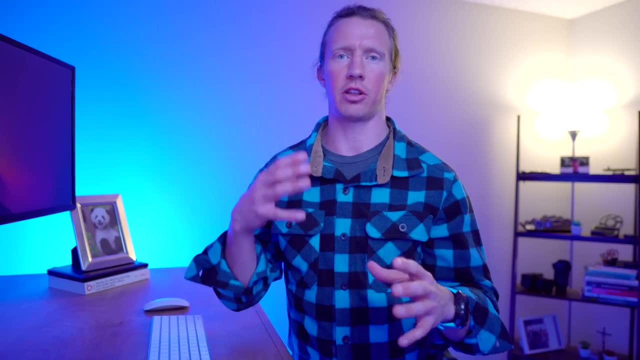 Personally, I've used Google Cloud Platform in the past, but many other options are just as good, especially AWS. Now, as an entry-level data analyst, I don't think you need to learn or master cloud providers. Instead, what I've seen is typically data engineers or even data. 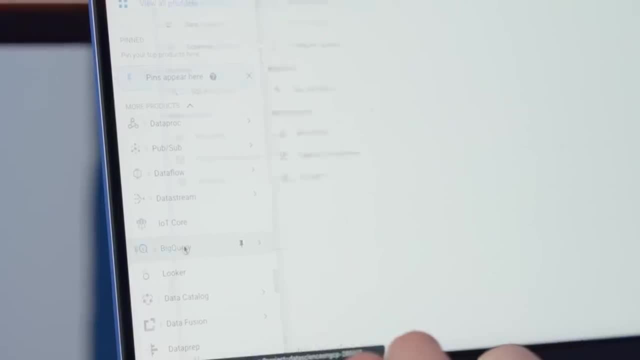 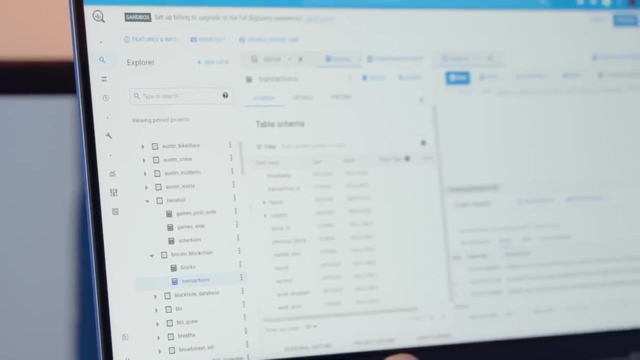 scientists are the ones setting up databases inside of some sort of cloud provider. However, it is important to know that these cloud providers provide some sort of interface for you to run SQL queries for your databases, As an example in the Google Data Analytics certificate. 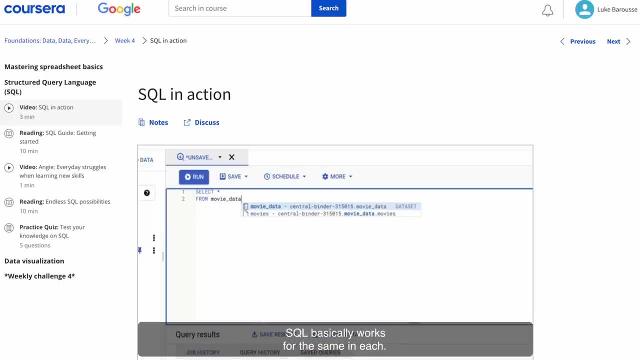 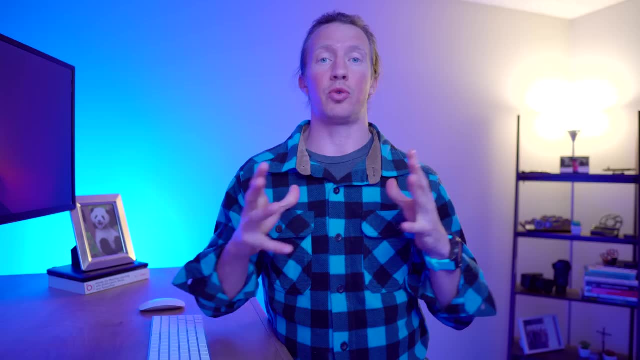 students use BigQuery inside of the Google Cloud Platform to run their SQL queries, And this actually leads into the next area of where you should be writing and running your SQL queries. Well, you could use a cloud platform in order to run your SQLs. 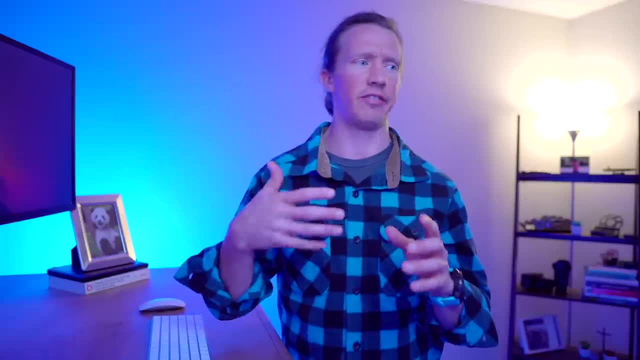 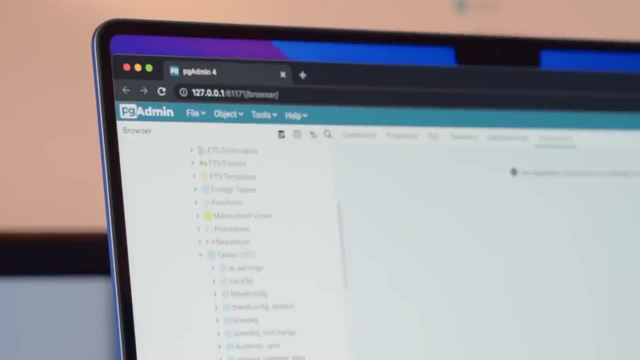 on those databases in the cloud. But what happens if you have a different environment or your database isn't in the cloud? All the major relational databases actually have their own editors for them. I've used Postgres before and for this I've used their SQL management software. 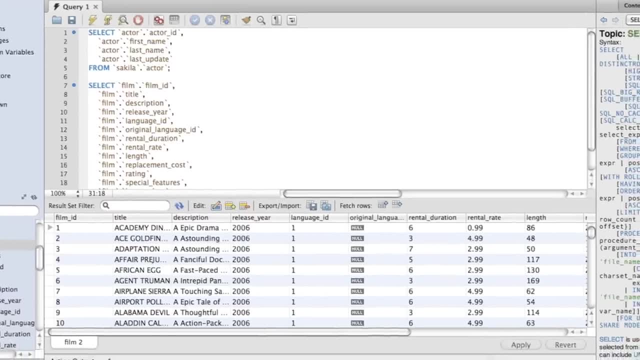 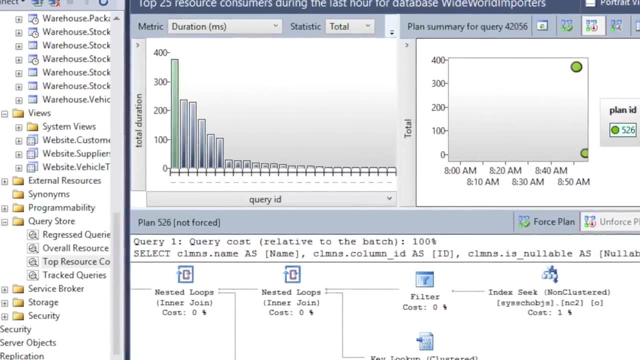 of pgAdmin. MySQL also has a similar software called MySQL Workbench to run their databases, And then for my work with SQL Server, I've even used Microsoft's SQL Server Management Studio. One note is that this tool is specifically only available for Windows users. 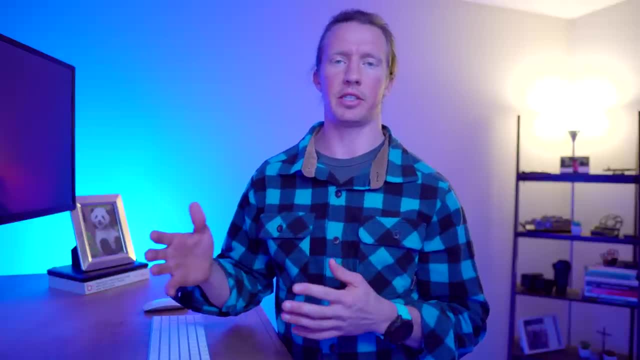 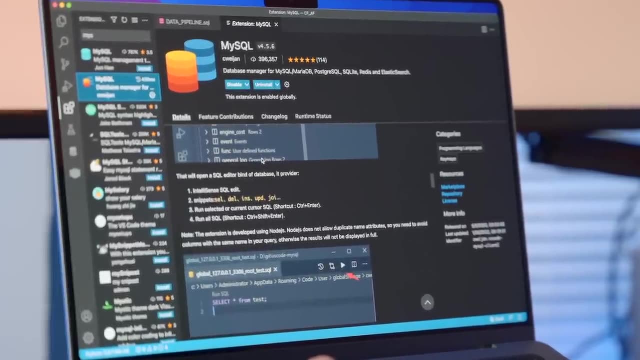 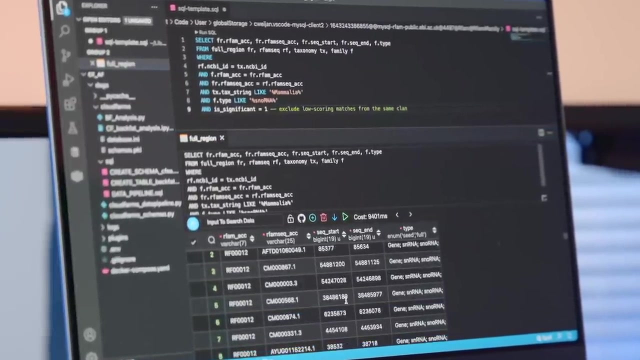 But what happens if you're like me and you're always switching between different databases? For this, I like to use VS Code. VS Code has many free extensions in order to support your database of choice. I'm currently checking out this extension called MySQL which, contrary to its name, actually supports a lot of the different popular databases. 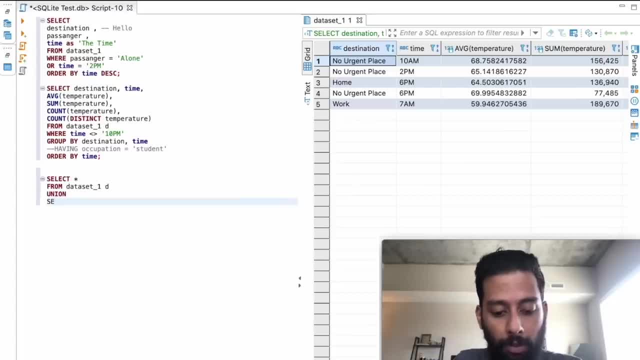 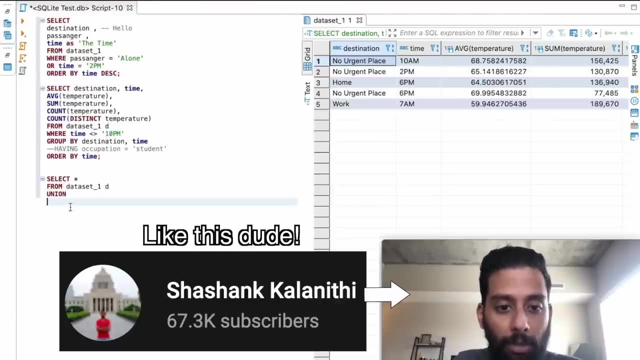 Another popular option to check out is dBeaver, So I haven't used this one personally, but it does seem like a good option, as recommended by other data analysts. Just like VS Code, it's free and supports a variety of different databases. 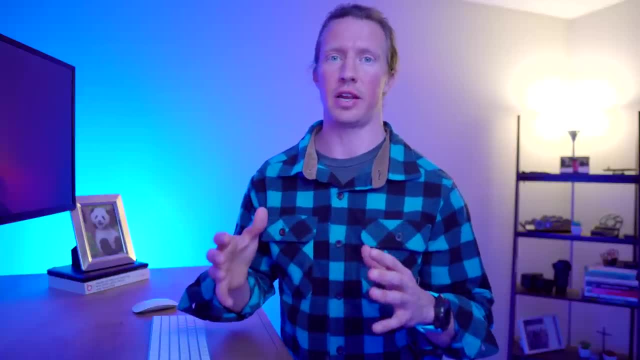 Now there is a lot of stuff that you can do to support your database of choice. There is one option that I don't suggest learning for those new to data analytics, and that is Microsoft Access. It's sort of a weird in-between of a relational 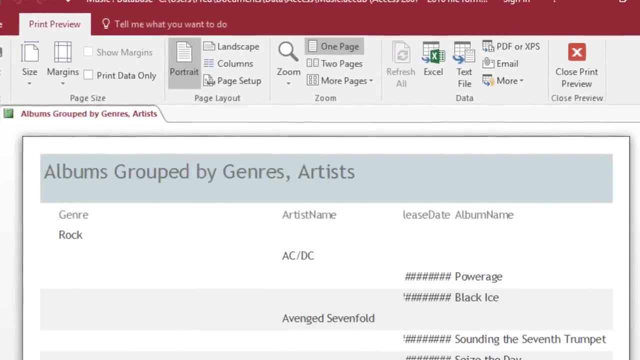 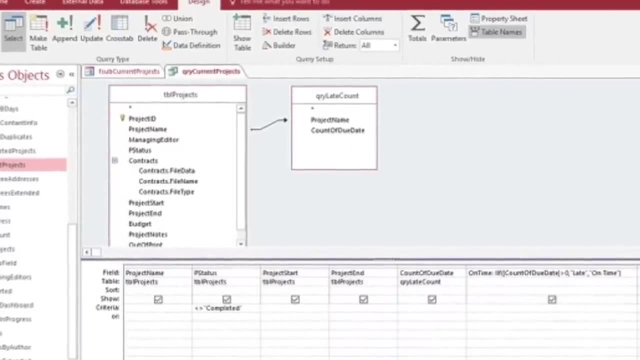 database and also a graphical user interface that you can build apps. We used this app while I was in the Navy in order to store our data, and the data nerds that worked with this were not really a fan of it. Now the reason why I'm recommending not learning this as a new data analyst. 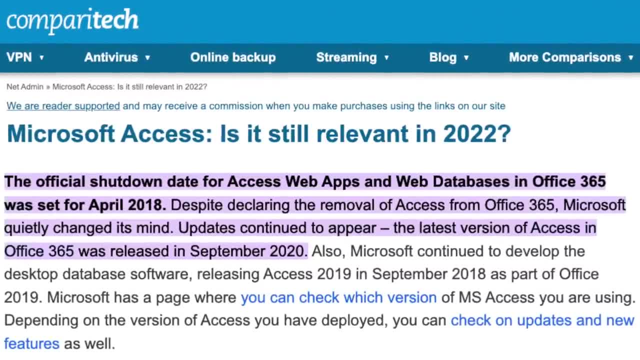 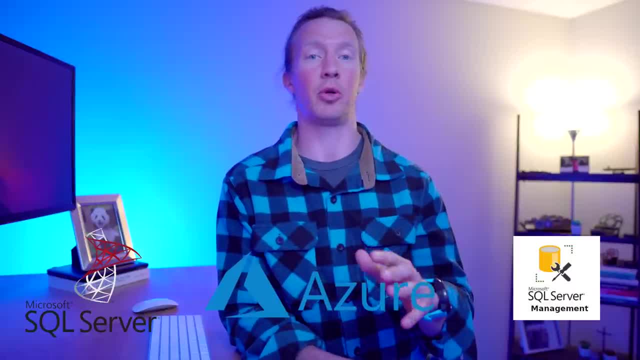 is because I feel Microsoft is actually signaling that they're going to be shutting this product down. So sorry to anyone that uses this product currently, but personally I feel Microsoft has way better options available in order to solve these types of problems. So, getting back into a real-world example, 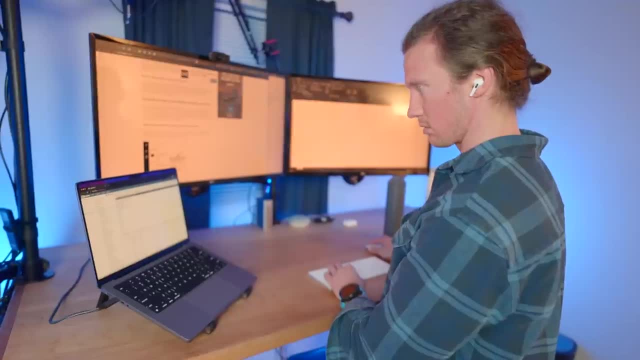 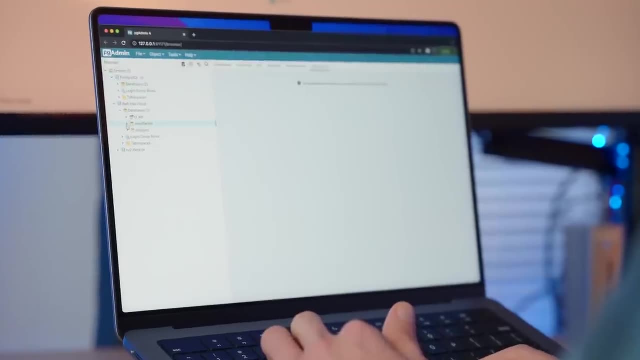 of how I use SQL in my job as a data analyst. So for one of my projects we needed to investigate the suppliers that we received a lot of our goods from for the company I worked for at the time. The problem is that the data was spread out across many tables within our database. 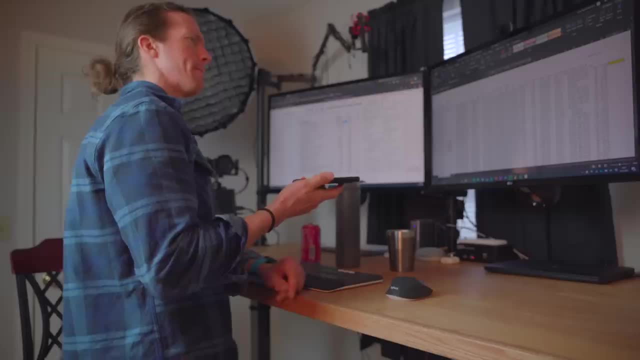 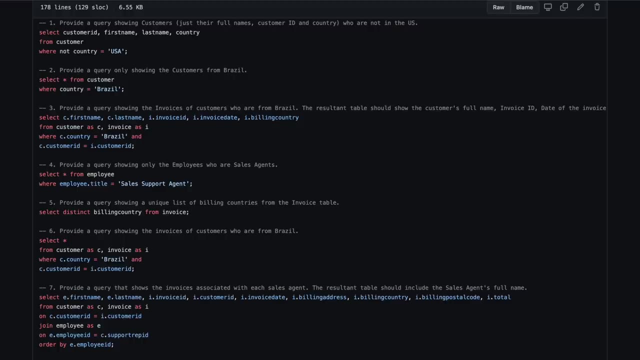 and required extensive cleaning. This was a large set of data, so a teammate and I worked together in order to build a SQL query to combine all these different tables that we needed and clean up the data. This portion of the project ended up taking a few weeks for us to actually 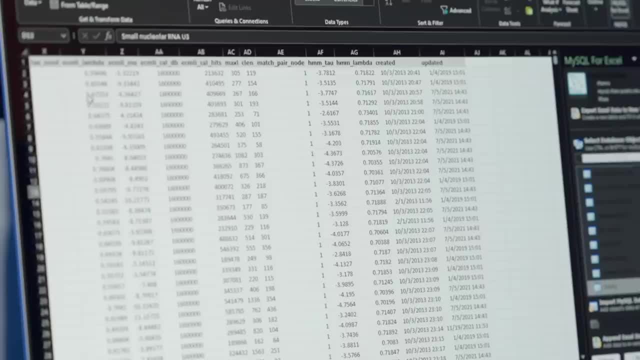 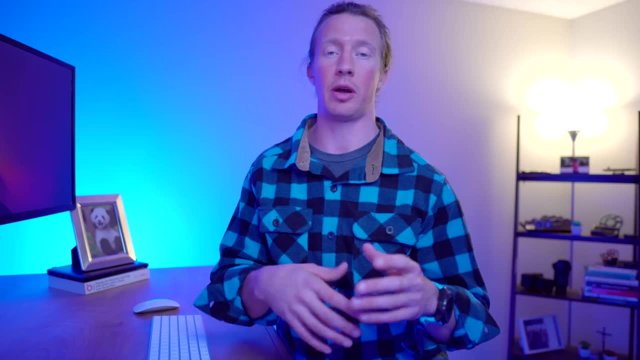 develop these few hundred lines of SQL in order to query this data. Now that we had this cleaned up data set, my boss now was like: hey, I need this data set in a more presentable form so that way my teammates can use it and also her boss could access it. 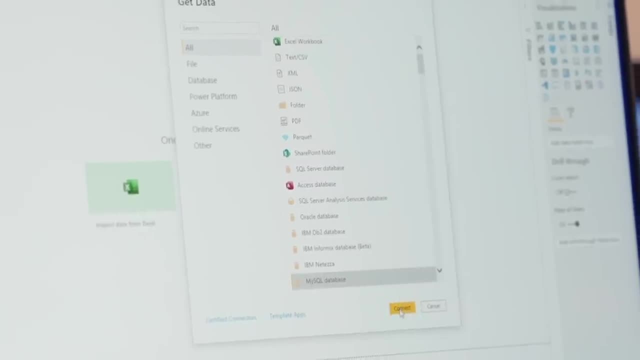 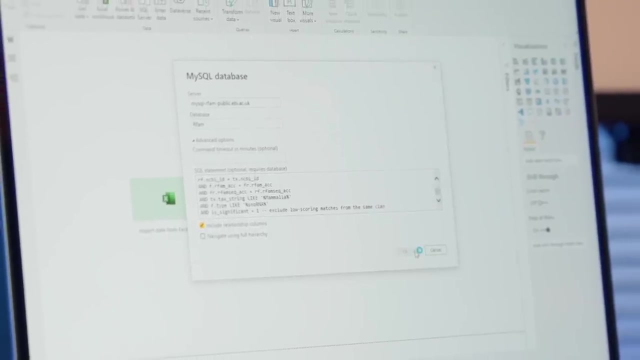 So that's where something like Power BI comes in. In this case, I can use the tool within it of Power Query, which is also in Excel, to actually go in and execute the SQL code we had written. And this is actually pretty neat because this allows the Power BI. 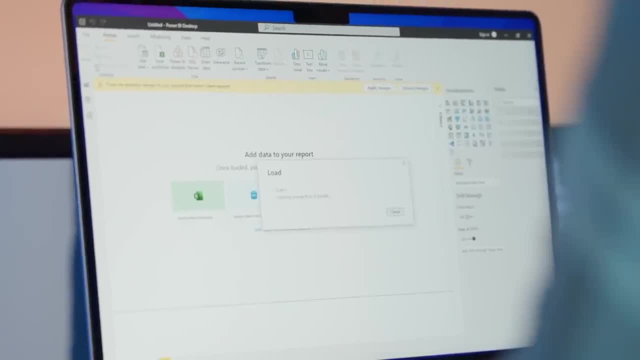 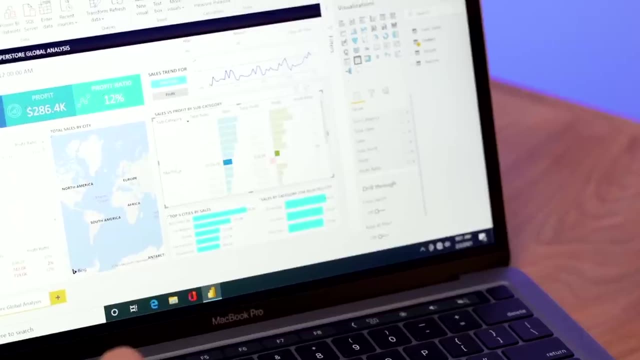 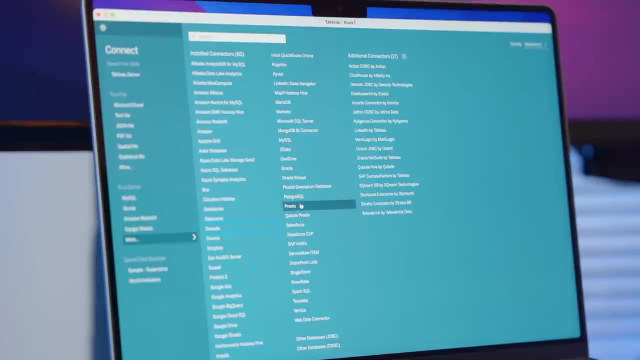 dashboard that we're going to build in order to be connected real time to the data source From here. I developed an end-to-end solution that allowed the stakeholders to now go to a dashboard and access the data that they were curious about. Now, to be clear, this SQL query functionality is not specific just to Power BI. Other popular 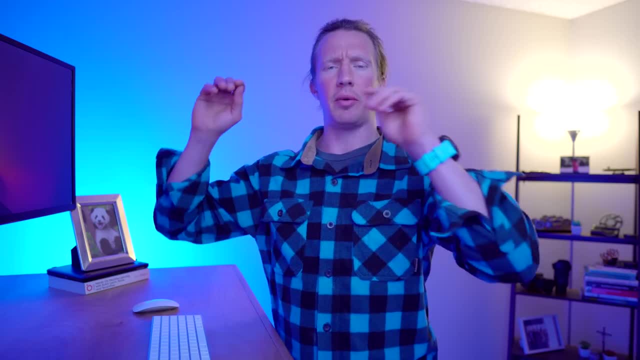 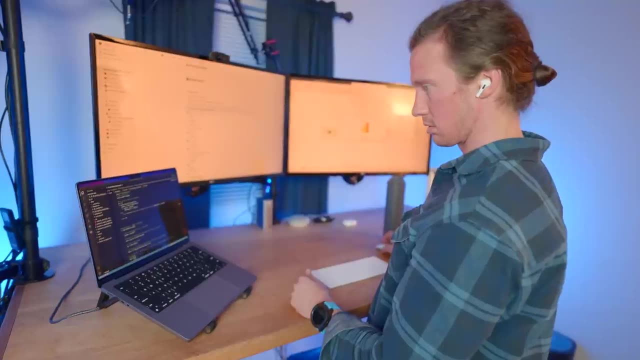 tools like Tableau and Google Data Studio also have this functionality. Now, not related to this project, but I've also used other tools, such as Programming, and I've also used this tool to program languages to utilize SQL as well. So, as I've mentioned before, I'm a big fan of Python. 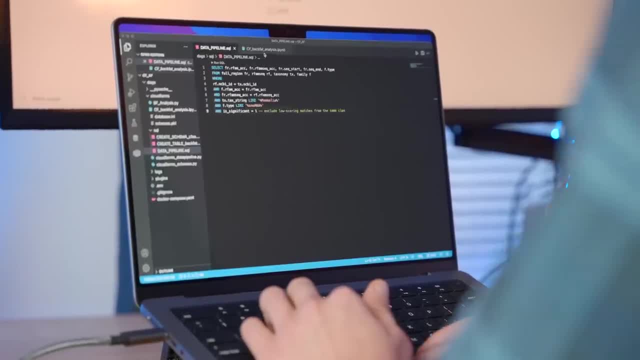 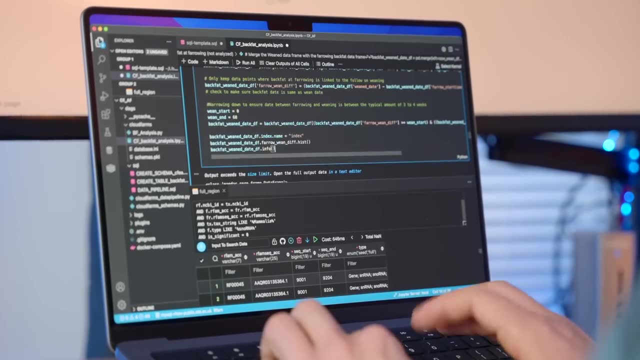 and I would say actually I'm more comfortable with Python than I am SQL. So a lot of times I like to get the data and then import it or collect it with Python And then from there use Python's tools and libraries, such as Pandas, to clean up the data. 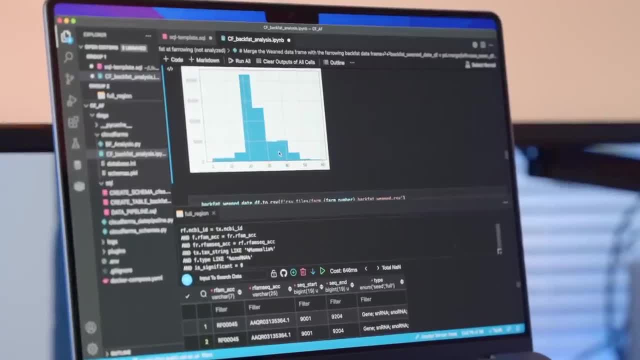 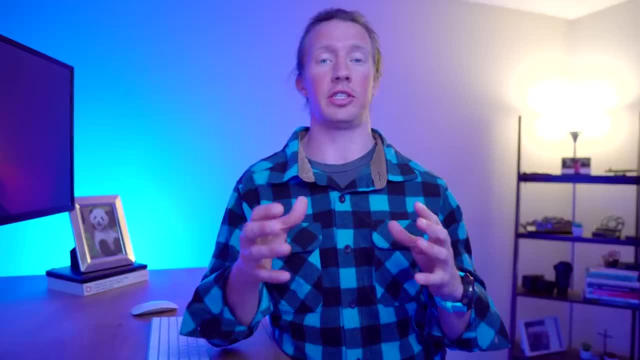 maybe Matplotlib to plot it and maybe something like sklearn to perform some regression analysis. Now, all these things with Python you can also do with other popular languages such as R also. So I share all these examples, not for you to think that you have to learn all.